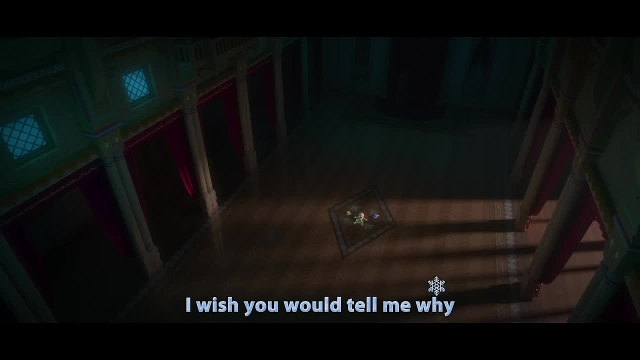 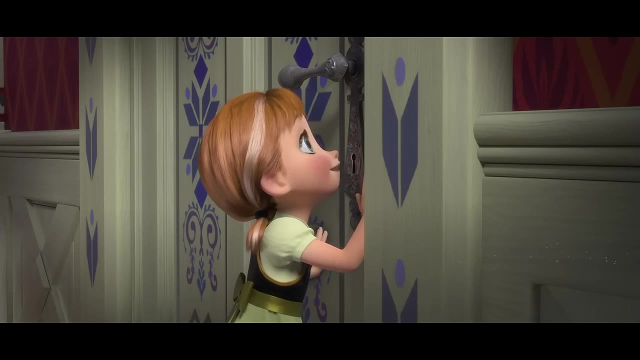 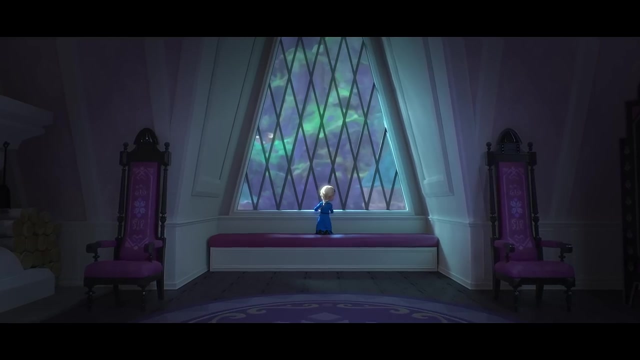 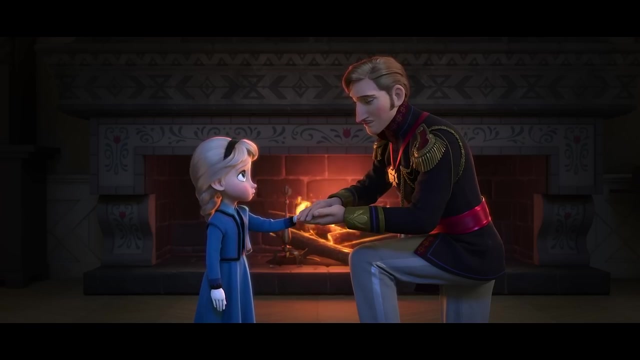 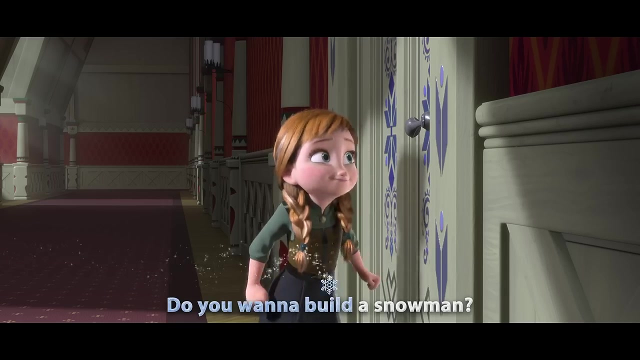 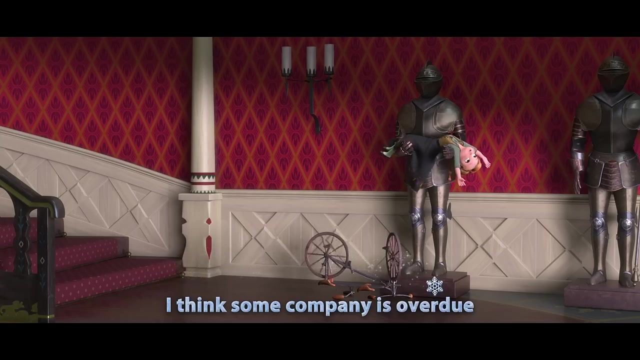 I wish you would tell me why Do you want to build a snowman? It doesn't have to be a snowman, Okay bye. Do you want to build a snowman Or ride our bike around the halls? I think some company's overdue. 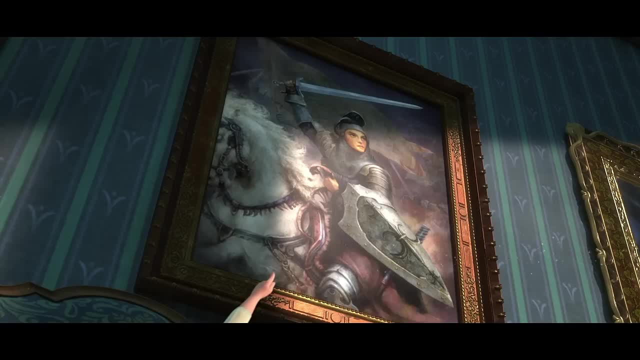 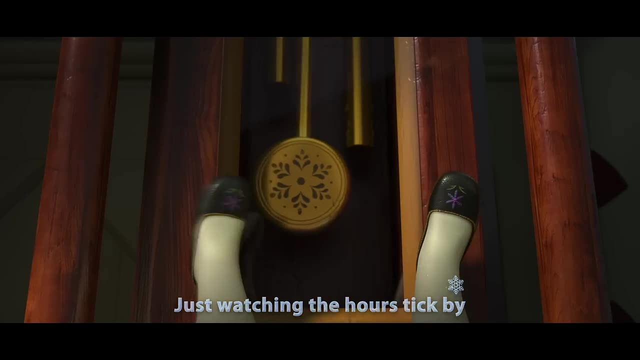 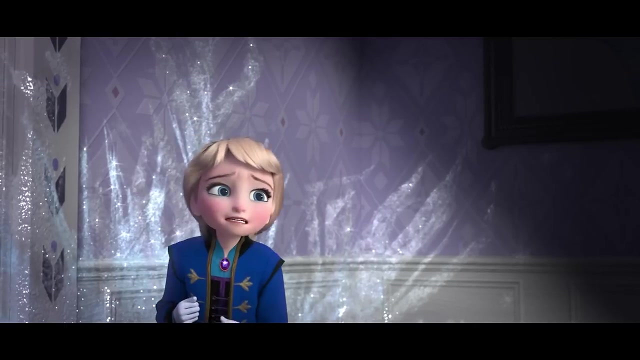 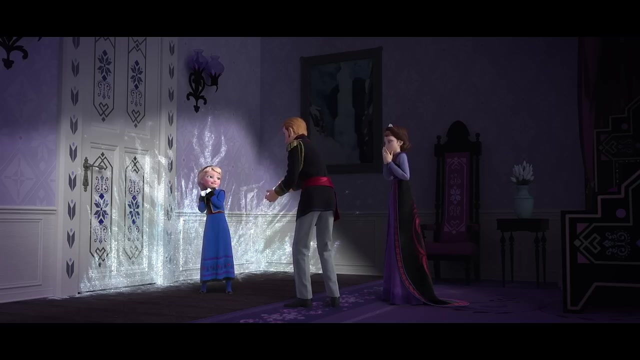 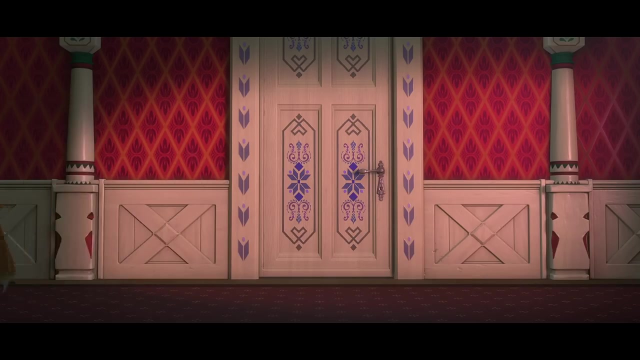 I've started talking to the pictures on the walls. Hang in there, Joan. It gets a little lonely all these empty rooms just watching the hours tick by. Come on, let's go See you next time. See you next time, Joan. 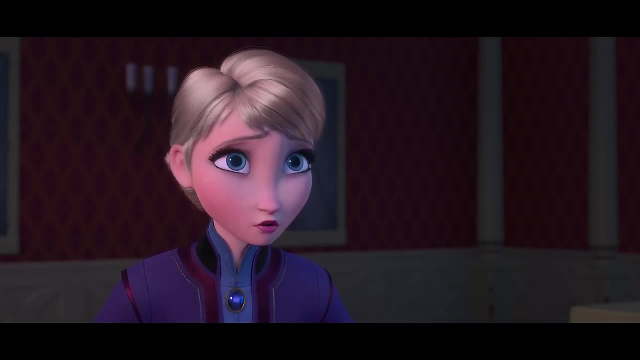 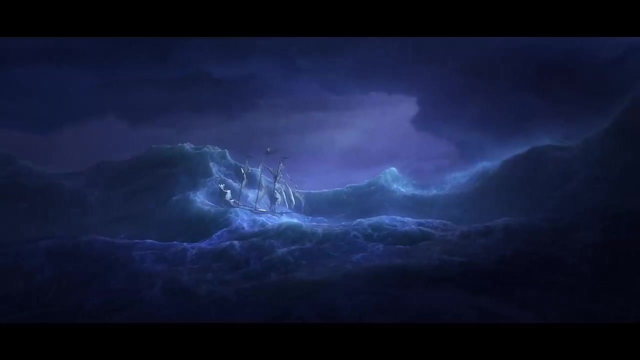 Ah, here I am. Oh, we're finally here. Oh, look at that. Uh-oh, Will we be able to pick up the snowman? I know this is not going to look that great, Yeah, but You didn't know. 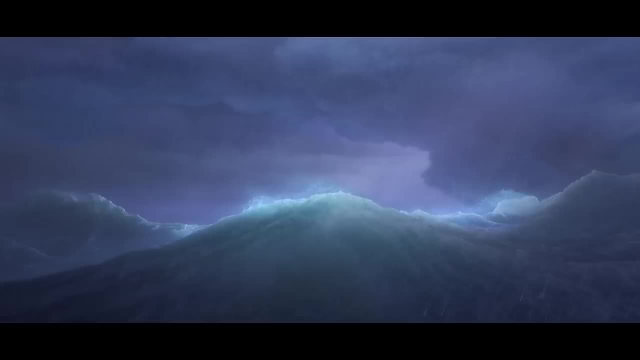 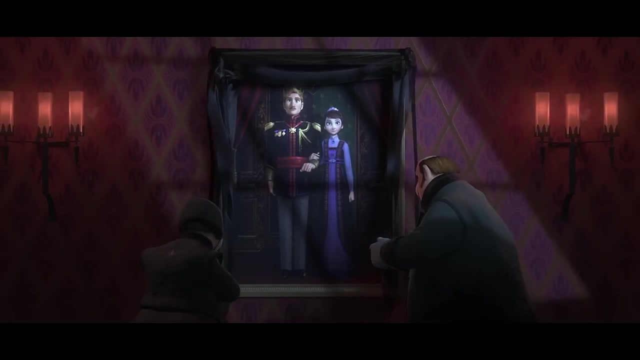 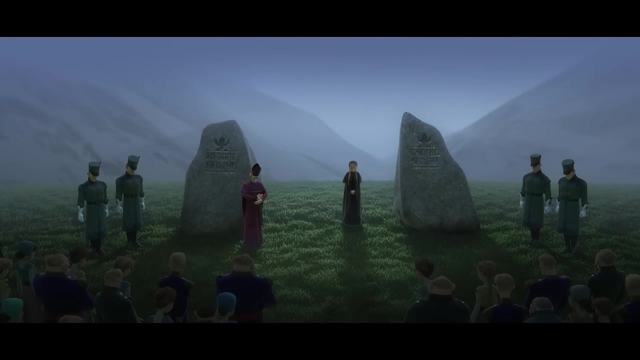 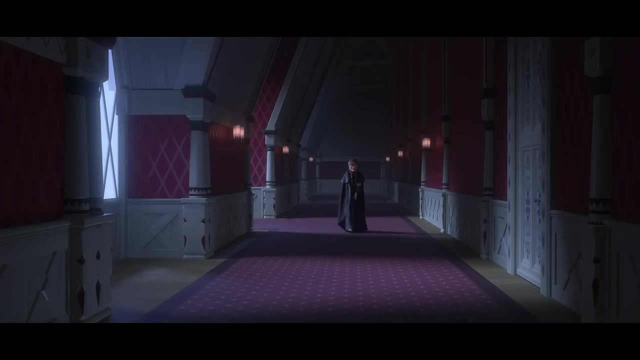 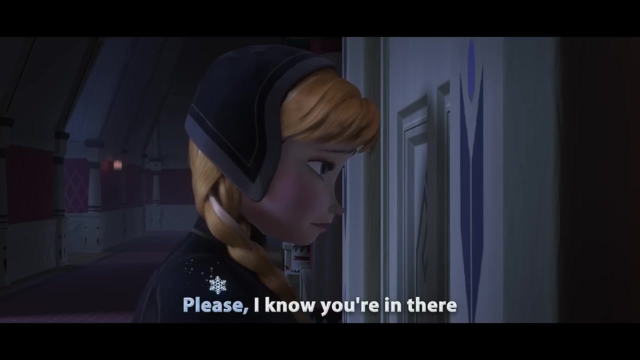 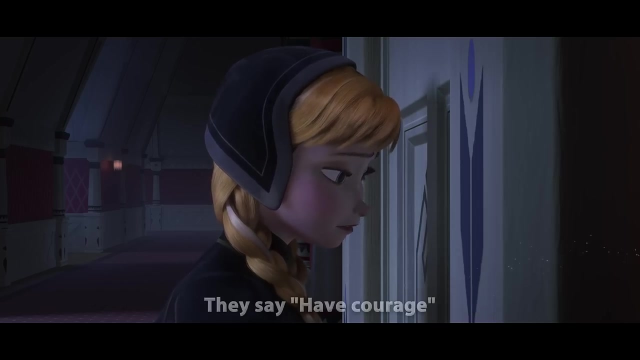 I said no. I said no. You said no, I love you. Uh, please, I know you're in there. People are asking where you've been. They say: of courage, and I'm trying to. I'm right out here for you. 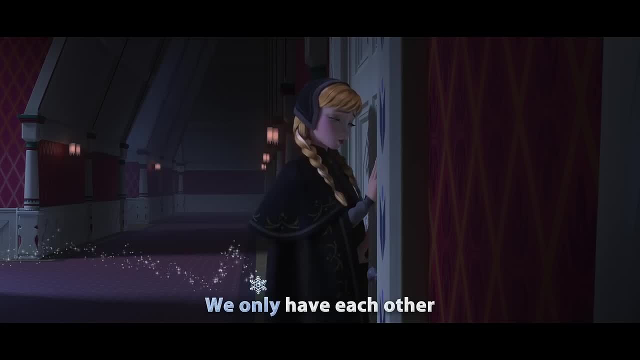 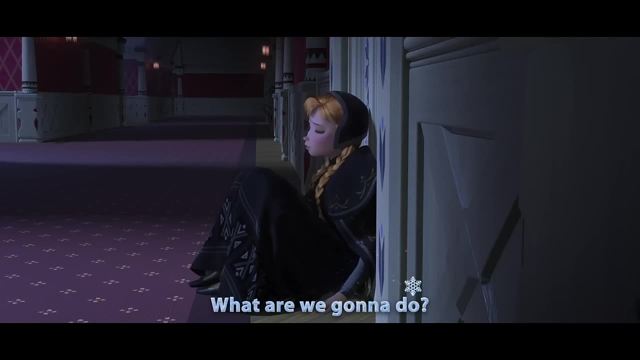 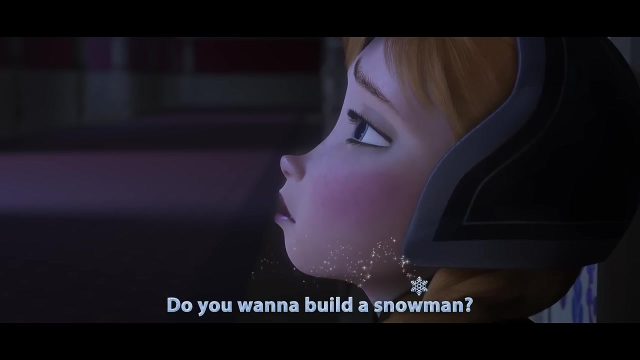 Just let me in. We only have each other. It's just you and me. What are we gonna do? Do you wanna build a snowman?